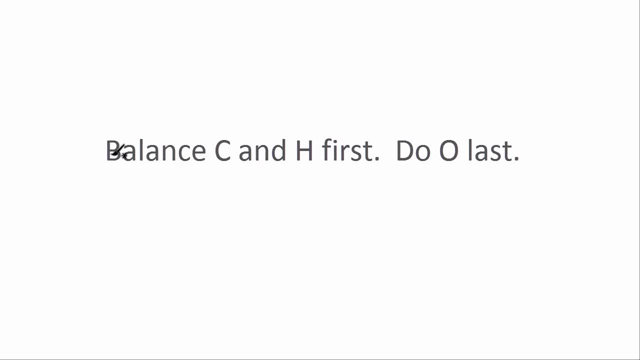 So deal with the carbons and hydrogens. first Use that fraction to fix the oxygens And then, if you want whole numbers, multiply all of the coefficients in the equation by 2.. So pause and try to balance this combustion reaction. 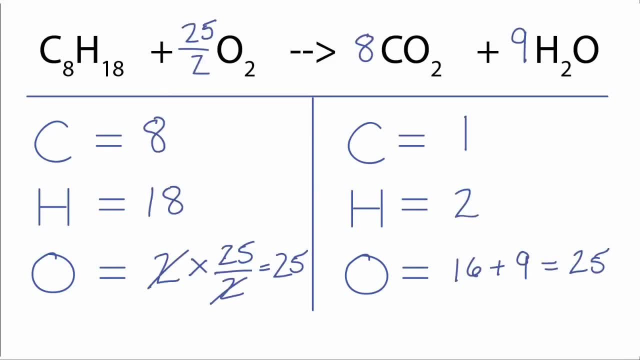 You should end up with something that looks like this: And then, if we wanted to have whole numbers in our coefficients, we could multiply the entire equation by 2. And that would give you coefficients of 2,, 25,, 16.. 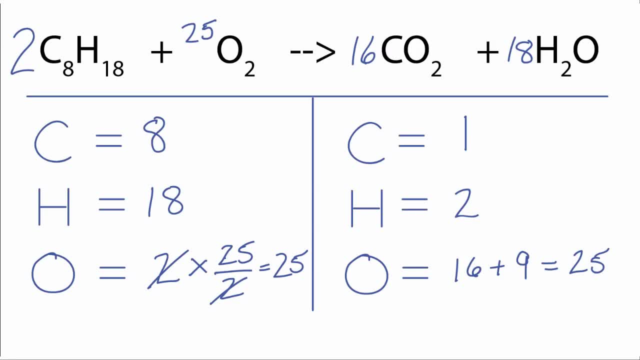 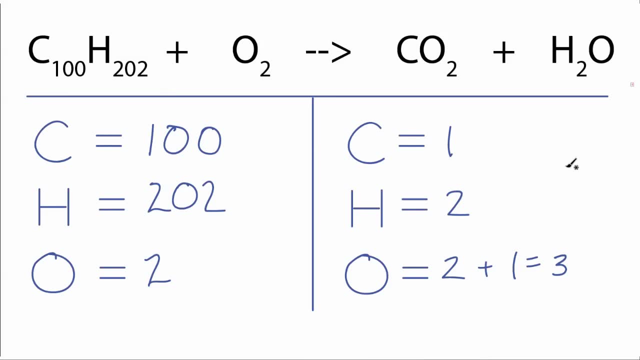 And 18.. Let's try one more, a little bit more challenging C100H202.. So pause and give this one a try. Let's balance this. We need 100 carbons over here, So 100 times the 1, that'll give me 100 carbons. 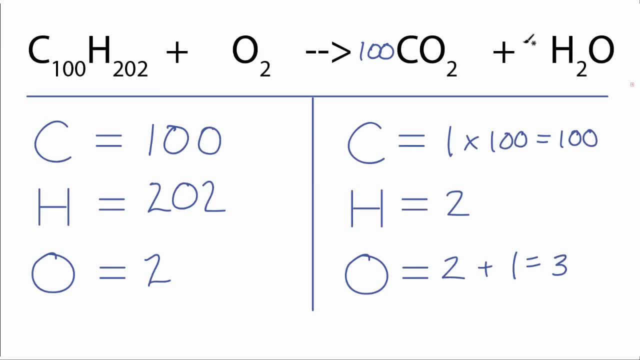 For my hydrogens I need 202.. So let's put 101 in front here, because 2 times 101 equals 202.. And now we need to recalculate our oxygens. I have 100 times 2, that's 200. 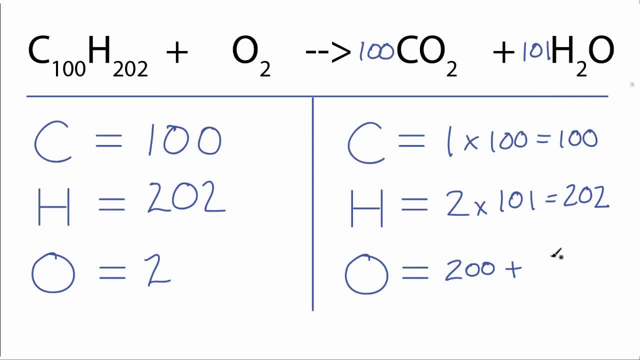 Plus 101 times the 1, that is 101.. So I have 301 oxygens to deal with. We know how to fix that. we just multiply this by 301 over 2.. And the 2's cancel out and we have 301.. 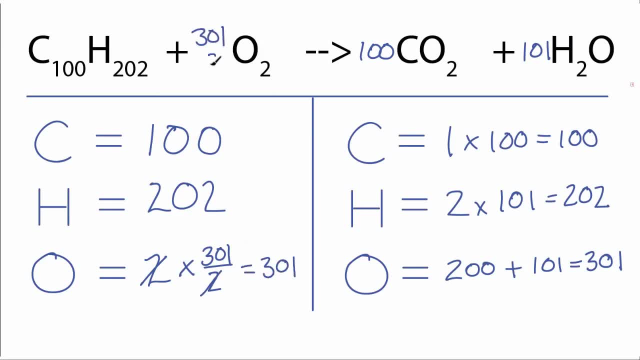 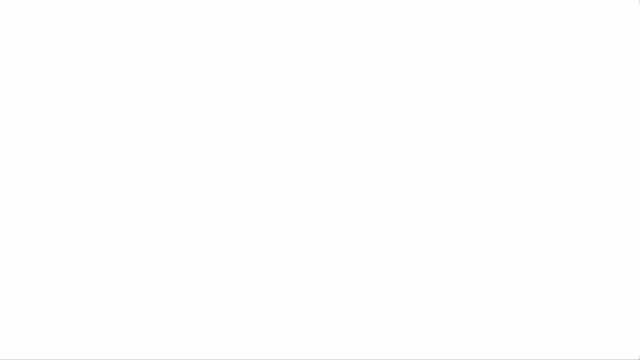 So we'll put our 301 over 2.. 301 over 2. here and now, this equation's balanced. If we want whole number coefficients, we can multiply the top of the equation by 2.. Again, the key to balancing combustion reactions. 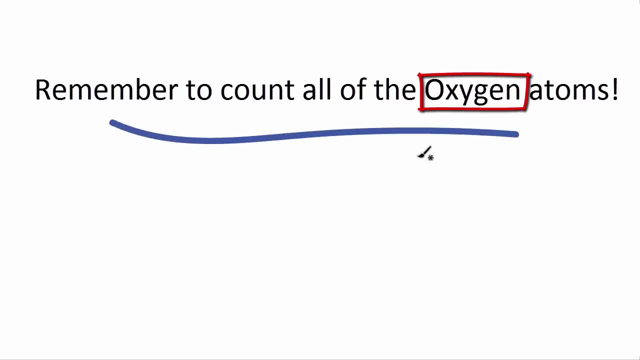 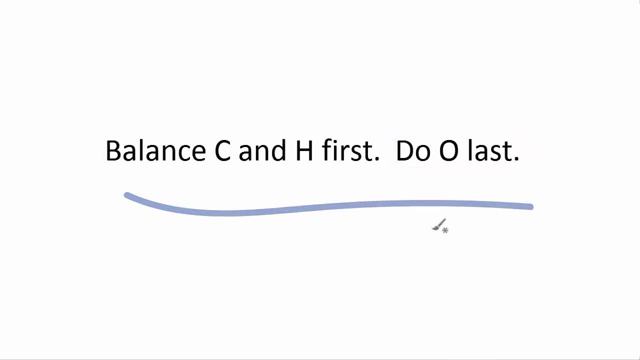 make sure you count the oxygens on both sides of the equations. Don't forget about the water. You then need to make sure that you do the carbons and hydrogens first, leaving the oxygens to last Use the fraction we discussed. 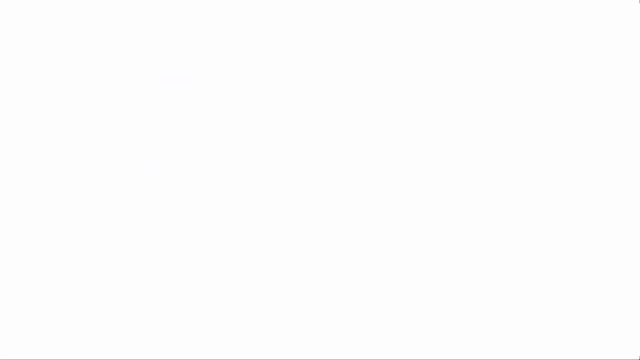 And then finally, if you want whole numbers, multiply the whole equation by 2.. This is Dr B and thanks for watching.